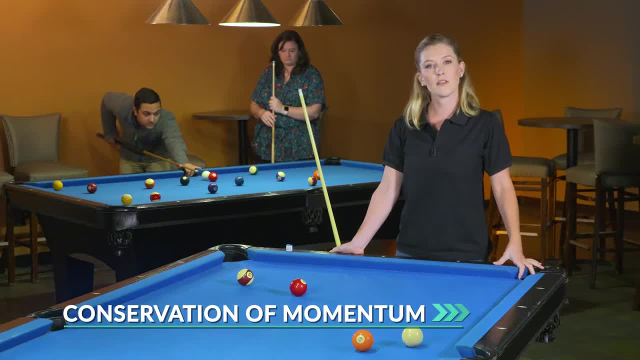 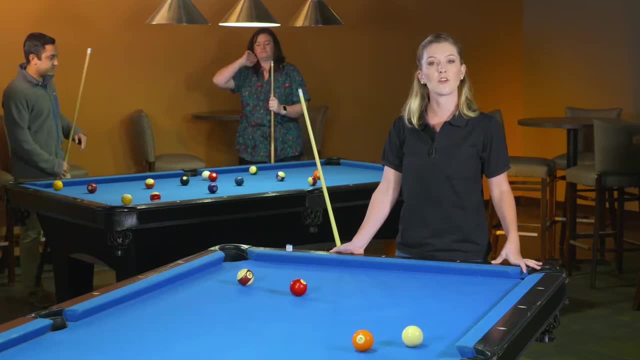 We'll find out how in this segment of Physics in Motion, as we look at the law of the conservation of momentum. During this series we'll talk about a few conservation laws specifically for energy, momentum, charge and mass. These fundamental quantities cannot be created. 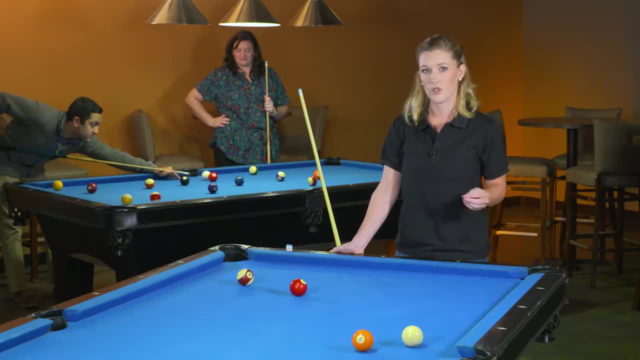 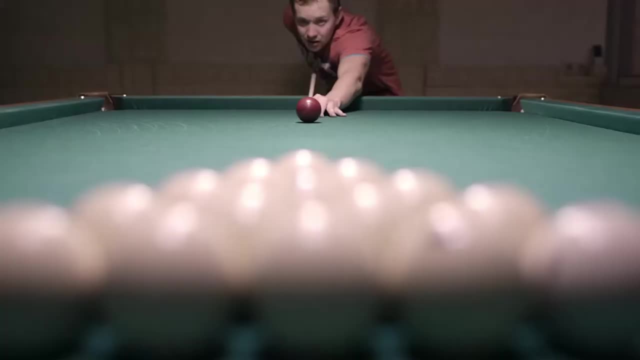 or destroyed. They can only be changed from one form to another or transferred from one object to another. So what do you think happens to the momentum of billiard balls when they strike another ball? If you figured that the momentum is conserved, you're right. The law. 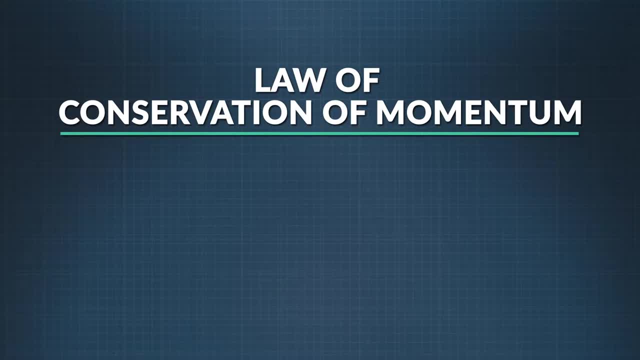 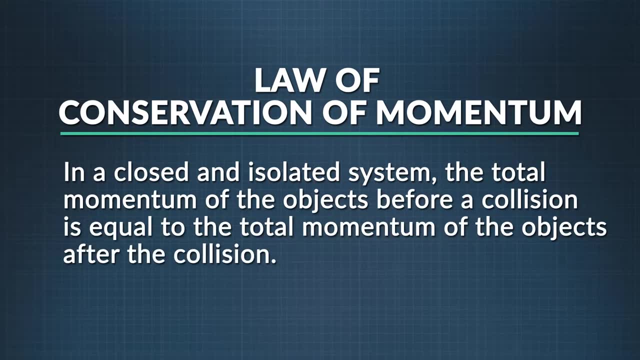 of the conservation of momentum says that in a collision between objects in a closed and isolated system, the total momentum of the objects in the system before the collision is equal to the total momentum of the objects in the system after the collision, Just like the other laws. 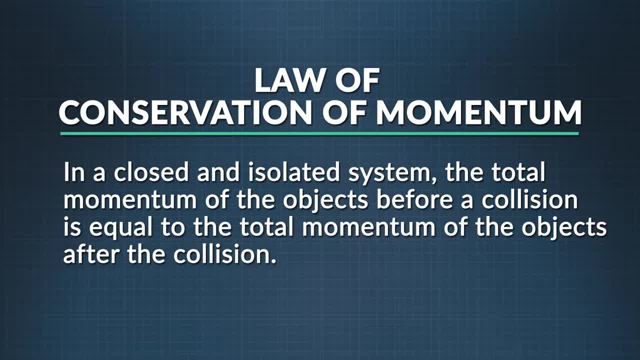 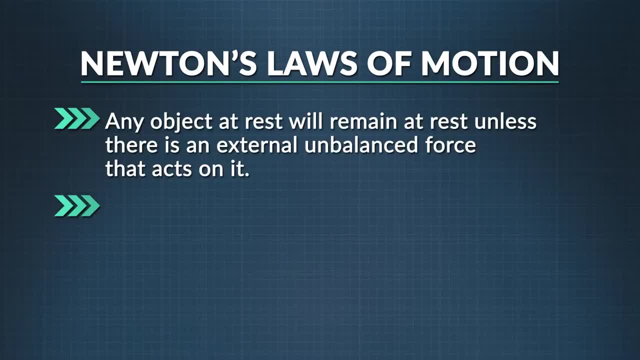 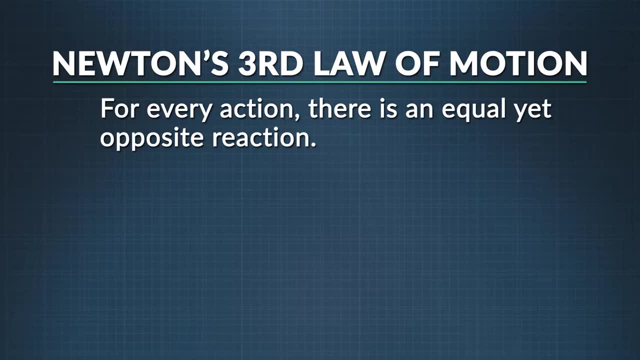 of conservation, momentum is not created or destroyed. There's another law of physics that might sound familiar when we talk about collisions, Remember Newton's laws, which predict the motion of most objects. His third law of motion states that for every action there is an equal and opposite reaction. 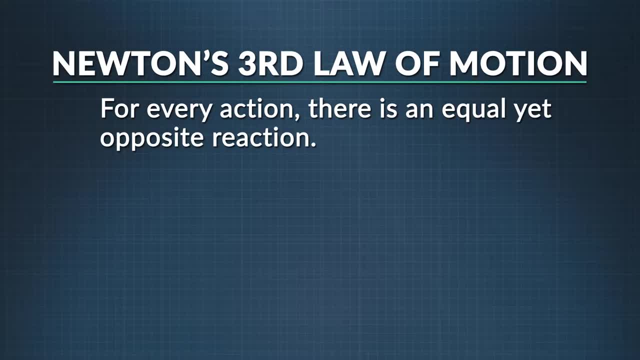 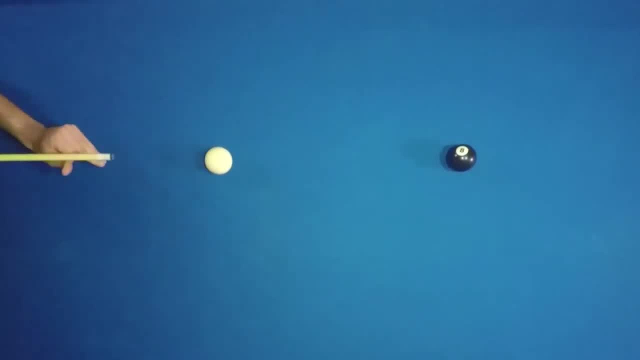 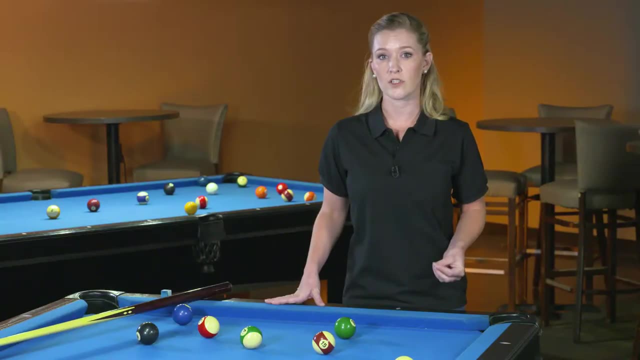 This means that objects exert equal forces on one another when they interact. One of the consequences of Newton's third law is the law of conservation of momentum. We can see it in action. when you hit a straight shot, and it does this, You exert a force on the. 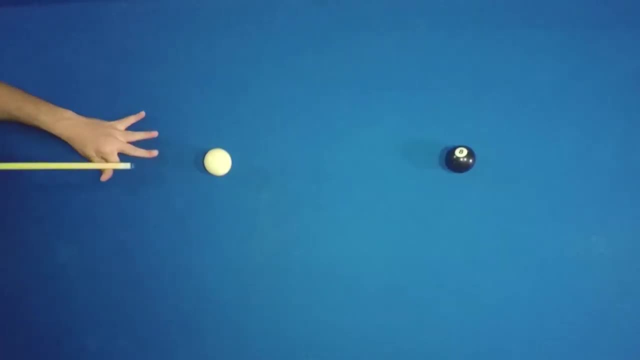 cue ball, which makes it gain momentum. When you strike the ball, that momentum is transferred to it. When the ball collides with the other ball—and the first ball stops—all the momentum has been transferred from the first ball to the second ball. 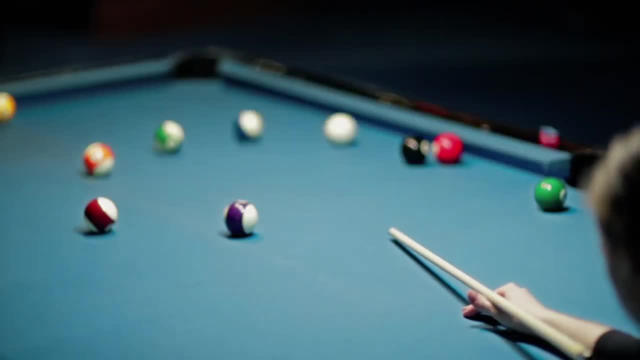 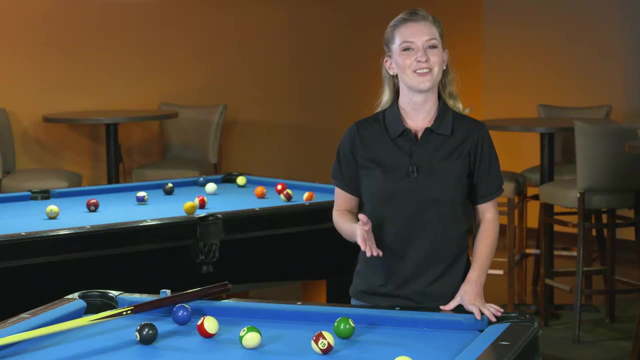 But what about in this case? This time the cue ball hits the other ball at an angle and both balls are moving. So was the momentum conserved? If you answered yes, you're right. Remember that momentum, like velocity and direction, is a vector quantity. 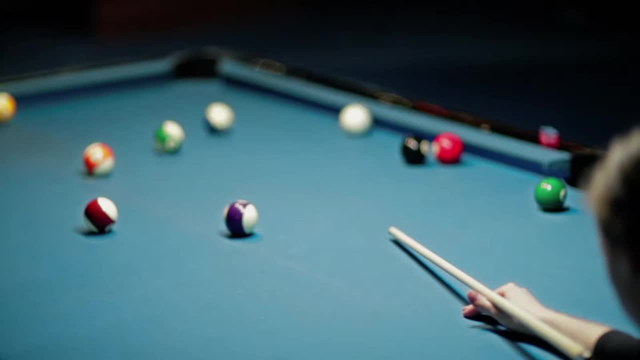 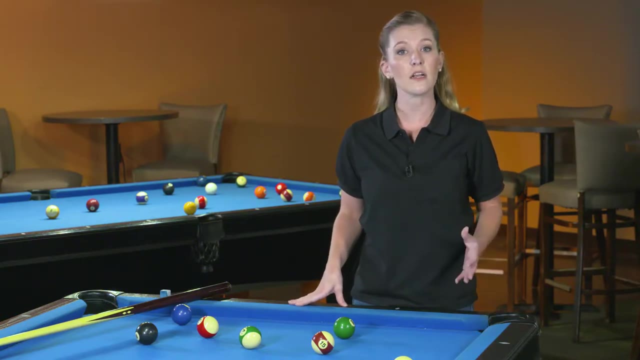 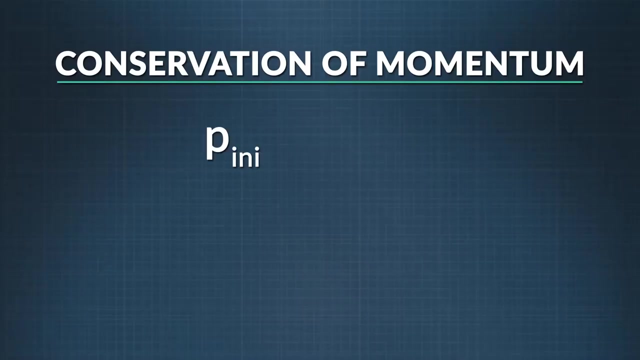 When the first ball travels in this direction, it carries some of the momentum with it. The rest is transferred to the second ball, but not enough to reach the pocket. However, none of the momentum was lost, only transferred. In equation form we see that the total momentum P, before objects interact with one another. 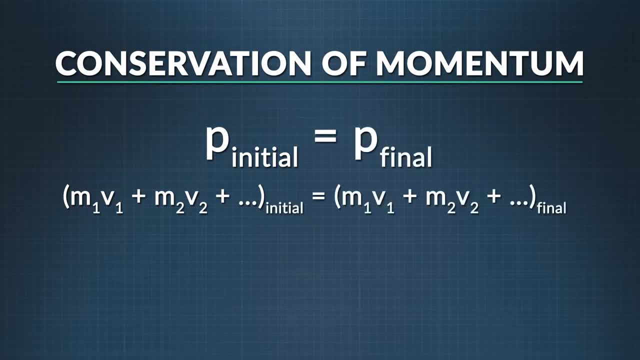 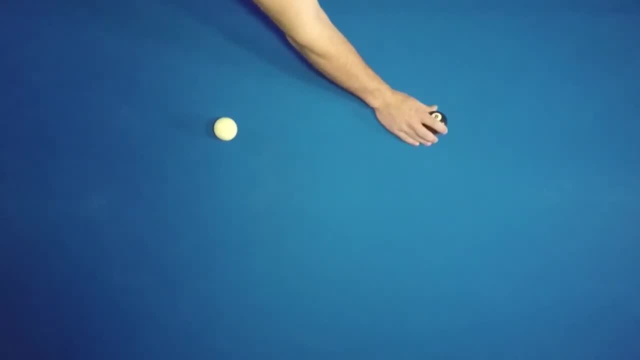 is equal to the total momentum of all the objects after they interact. Now, ready to try solving a problem, A pool player is about to use the cue ball to make a direct hit on the 8 ball, which is at rest. Each ball has a mass of 170.0 grams and the cue ball's initial speed is 6.00 meters. 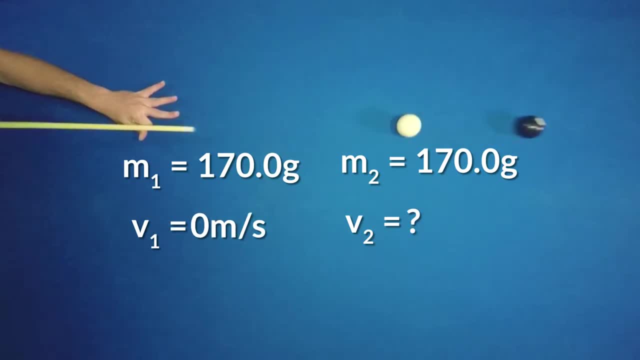 per second After the collision, the cue ball comes to a stop. If no momentum is lost in the collision, what is the total momentum of this system and how fast is the 8 ball moving after the collision? Remember, the momentum of an object is equal to its mass times its velocity. 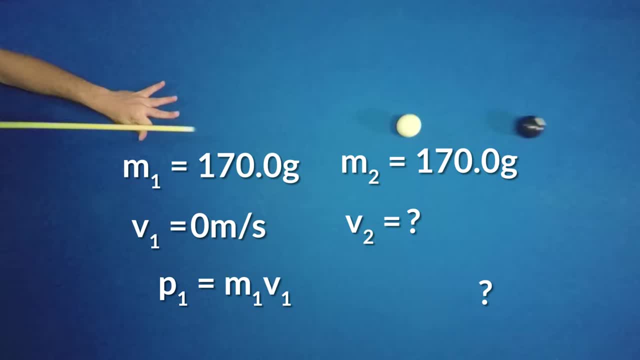 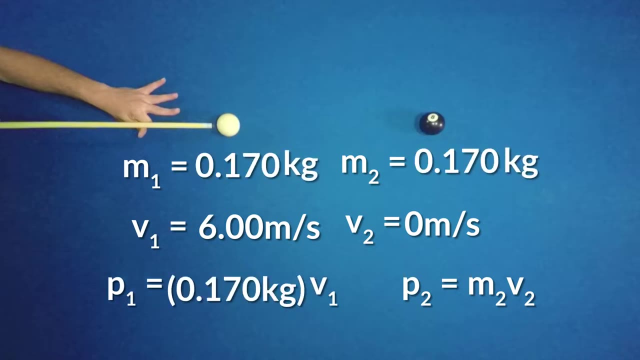 P equals m times v. The unit for momentum is kilogram meters per second. To be consistent, we'll convert the mass to kilograms. The cue ball has a mass of 0.170 kilograms, so let's multiply that by the velocity of. 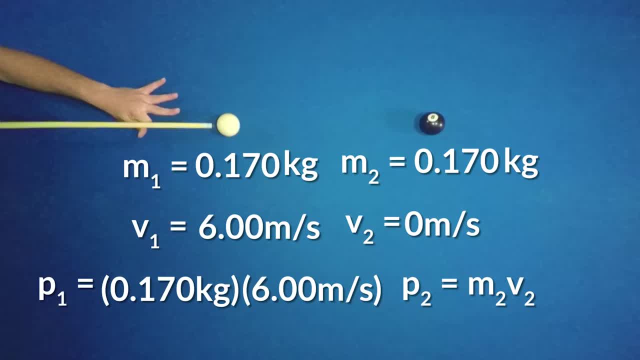 6.00 meters per second. So the momentum of the cue ball before the collision is 1.02 kilograms meters per second. Since objects at rest do not have momentum, the 8 ball begins with zero momentum. So the total momentum of the cue ball and the 8 ball together before the collision is: 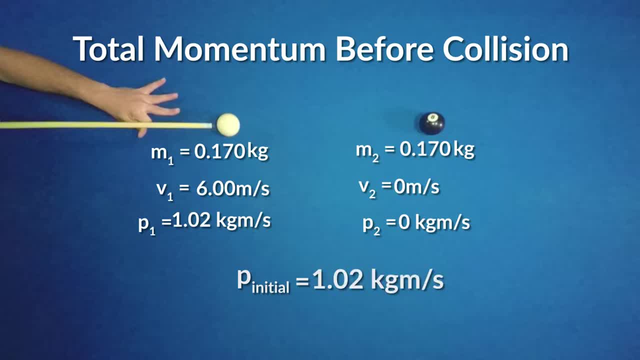 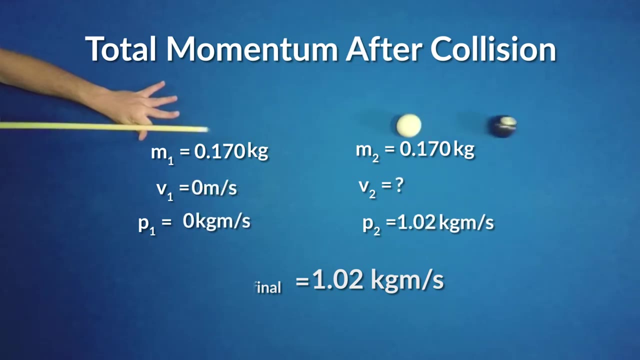 also 1.02 kilograms meters per second. And because momentum is conserved, 1.02 kilograms meters per second is the system's total momentum after the collision too. Now, what about the final velocity of the 8 ball? Since the collision brings the cue ball to 0.00 meters per second, the system's total momentum after the collision is 1.02 kilograms meters per second. 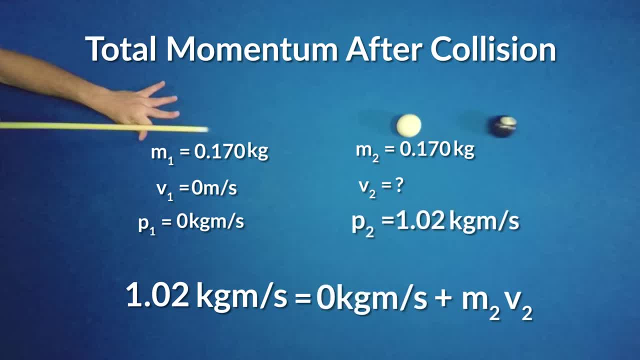 The 8 ball carries all the system's momentum. That means we can divide 1.02 kilograms meters per second by 0.170 kilograms, the 8 ball's mass, to find its velocity, And that turns out to be 6.00 meters per second, the same as the cue ball had at first. 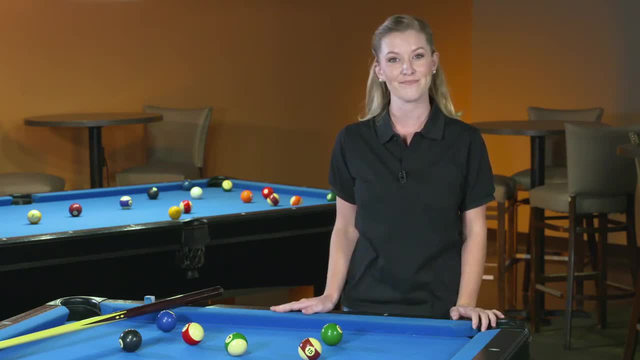 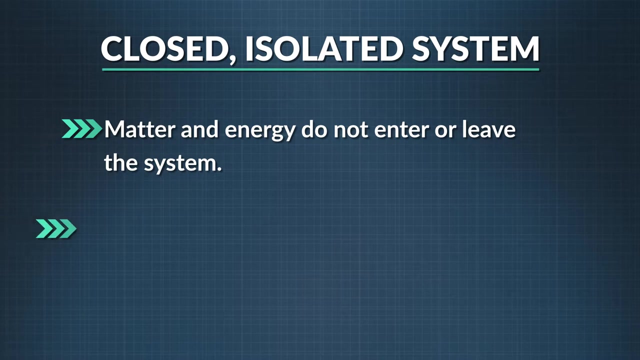 See how the law of conservation of momentum helped us solve this equation. You apply the law of conservation of momentum. You apply the law of conservation of momentum only when a collision happens in a closed, isolated system. That means matter and energy do not enter or leave the system, which means there are 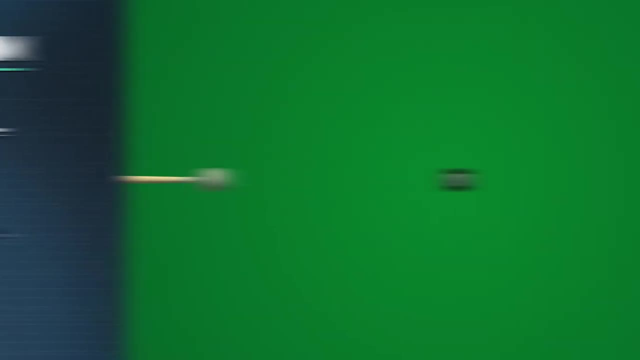 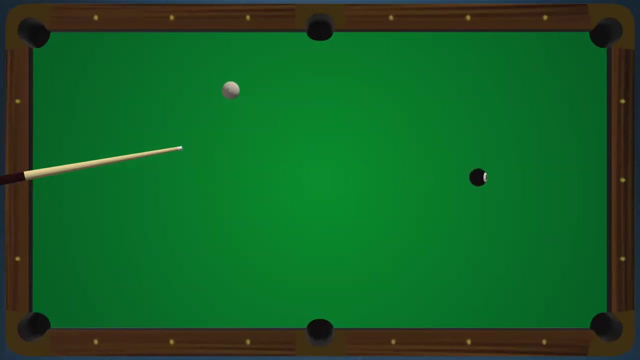 no net outside forces acting on the system. In our example, the two pool balls are the system. They don't enter or leave, so the system is closed. The only force we consider is the force between the two balls when they collide. We're not concerned about the initial force of the cue stick or the friction between the 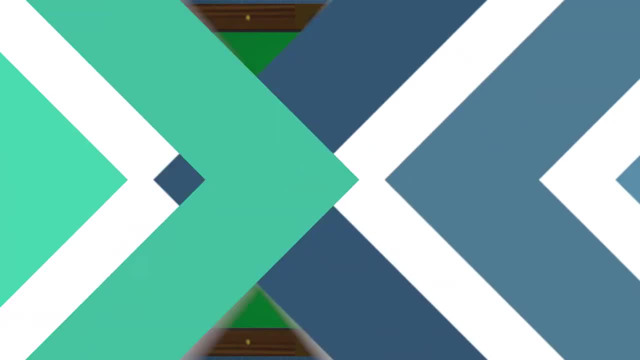 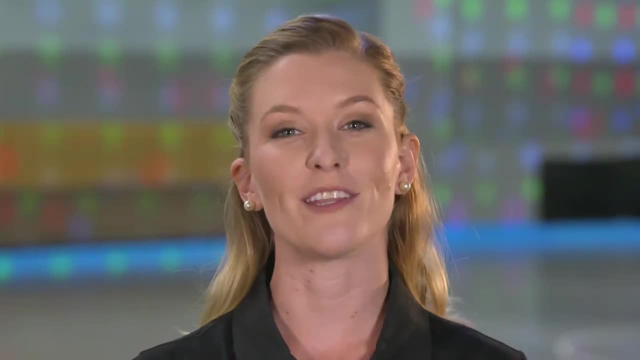 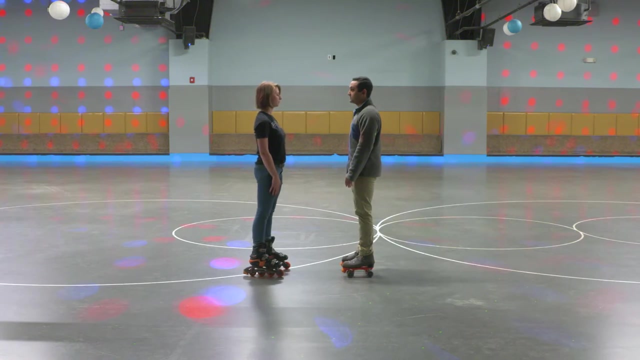 balls and the table. so we say that the system is isolated. Let's do one more where we can look at speed and direction, but this time we'll do it while roller skating. We have two people facing each other: Turag is 60.0 kilograms and Summer is 45.0 kilograms. 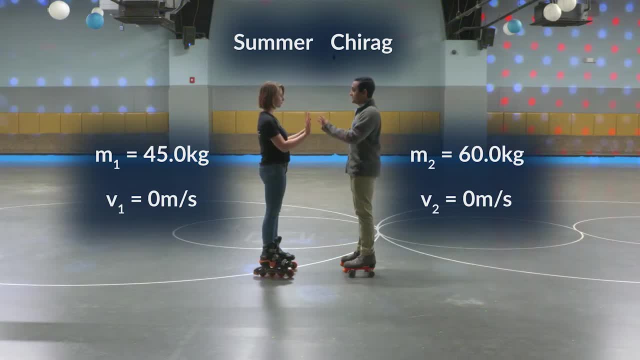 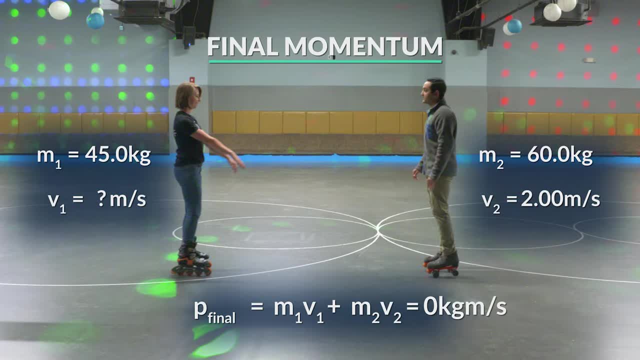 Caragues had a final velocity of positive 2.00 meters per second and Somers was negative 2.70 meters per second.